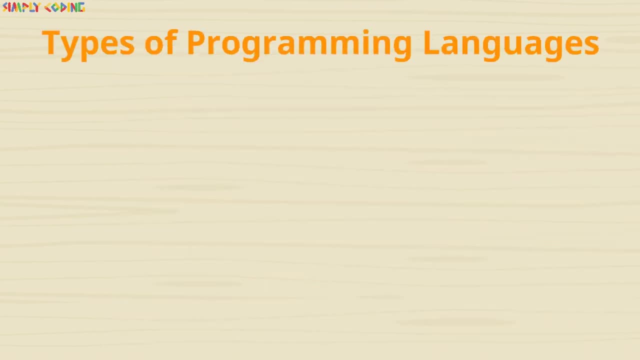 There are different types of languages. The programming languages are divided into two types: low level and high level. Low level is a language which machine understands and is of two types: assembly and machine language. High level languages are more user friendly and closer to human language. 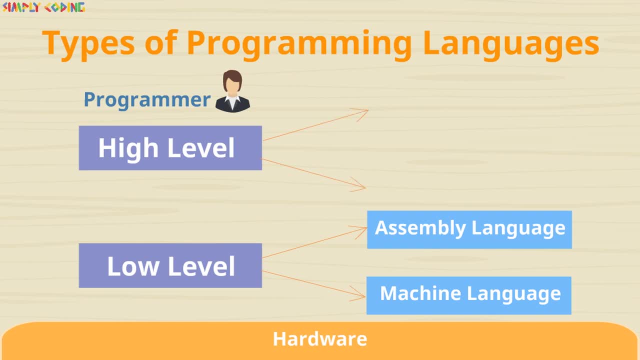 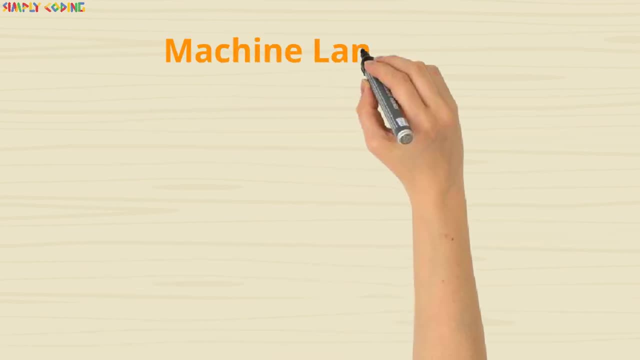 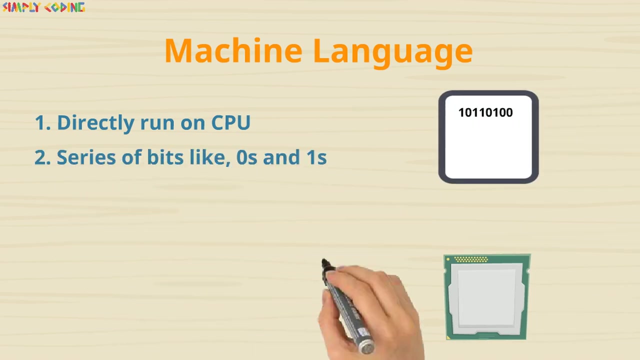 They are of two types: procedural and object oriented. Let's learn more about each of them. Machine language is the language which can directly run on CPU. They are numeric, That means in series of bits which are zeros and ones representing instructions that a computer can understand. 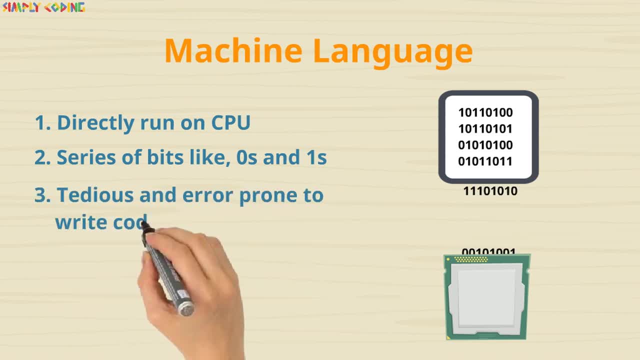 This makes it tedious and error prone to write machine code manually. They are not portable Means. a machine language is specific to a particular type of machine only. Ultimately, all languages need to be translated to machine language. On top of it, we have assembly language. 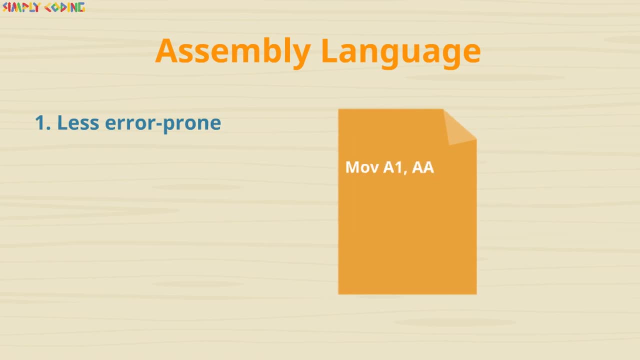 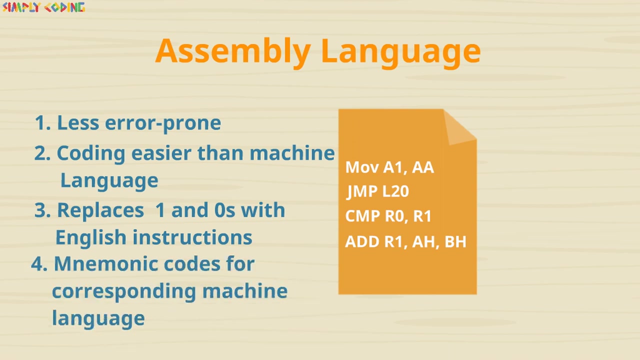 Assembly language helps eliminate much of the error prone and time consuming machine language programming. It replaces remembering one and zeros with instructions which are mnemonic codes for corresponding machine language Example. it has commands like move, jump, cmp, add, etc. Each assembly language is specific to particular computer architecture and sometimes to an operating system. 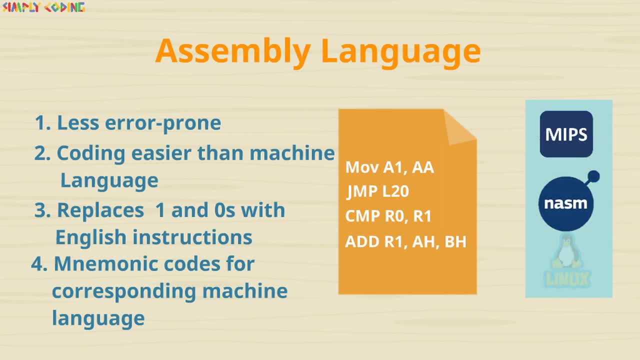 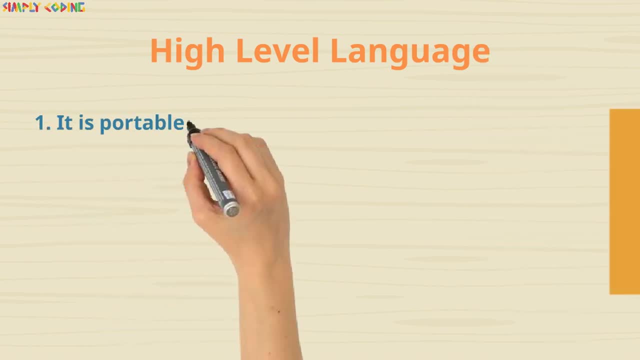 Examples include MIPS, NASM, x86, etc. Now let's take a look at high level languages which are portable and statements are in English, like language making it convenient to use. These include C, sharp, Java, Python, etc. The amount of assembly language is very important. 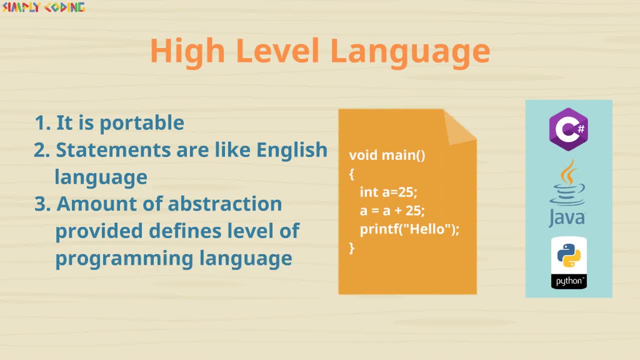 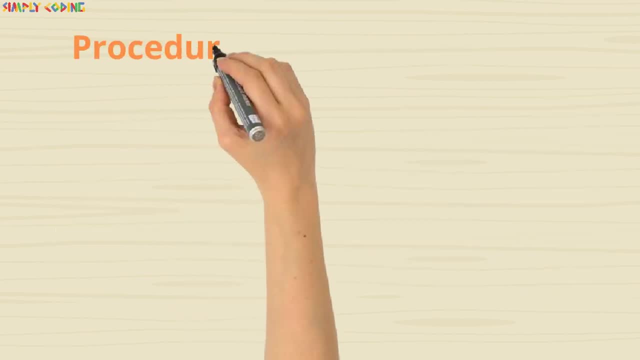 The amount of abstraction provided defines how high level a programming language is. The high level languages are also of two types: procedural language and object oriented language. In procedural language, the program is written in terms of sequence of steps to solve the problem, For example, steps given in a recipe or sequence of steps you follow when you wake up.